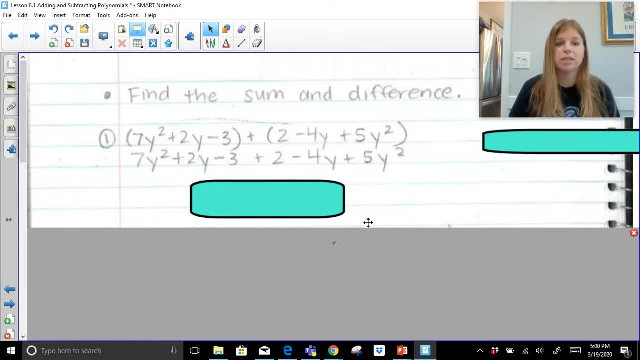 highest exponent to the lowest exponent. So when I look at this I have 7y squared plus 2y minus 3 plus 2 minus 4y plus 5y squared. The highest exponent, the highest degree here, is 2.. So I'm 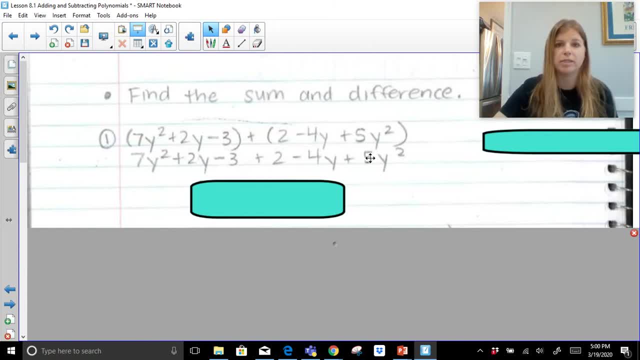 going to look at my 7y squared plus 5y squared and I'm going to add those together first. 7y squared plus 5y squared would give us 12y squared. Remember when you're adding like terms, you're. 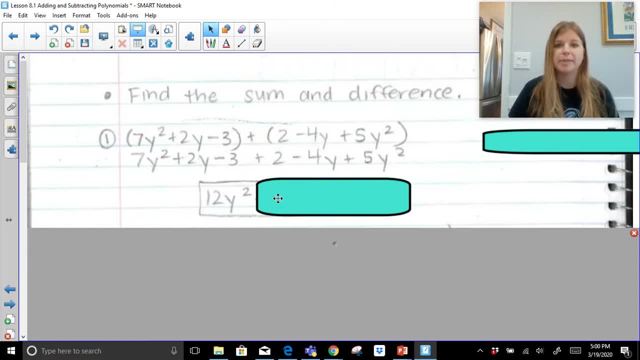 just working with the common denominator, So I'm going to add those together first. So the exponents are just going to change. I always say in my students: what's 2 oranges plus 3 oranges? You would say 5 oranges. You would never say 5 oranges squared or 5 oranges to the 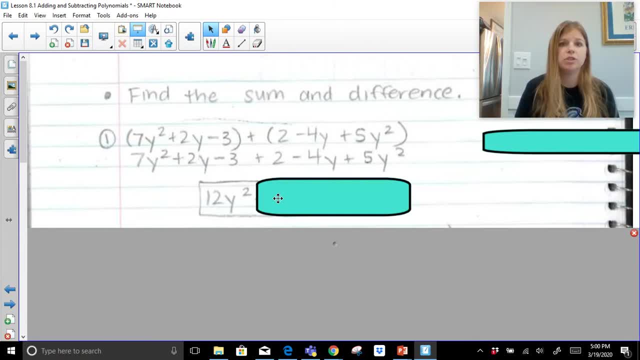 third power: You would just leave it. So then, if 2x plus 3x is 5x, then 2x squared plus 3x squared is 5x squared. The exponent stays. you're just working with the coefficient. Next, after I deal: 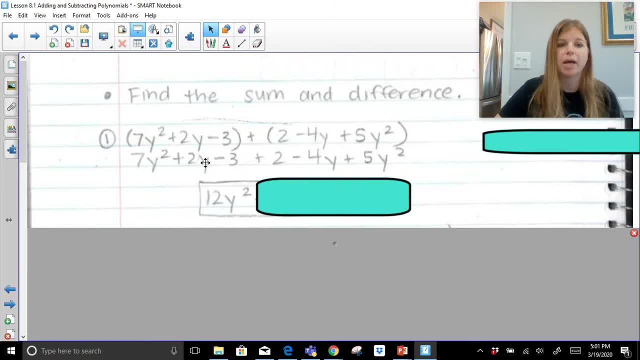 of my squares. I will look at my exponent of 1.. I've got a positive 2y and a negative 4y. Positive 2 minus 4 is a negative 2y. Lastly, I looked at my constants, which are just my numbers. A negative: 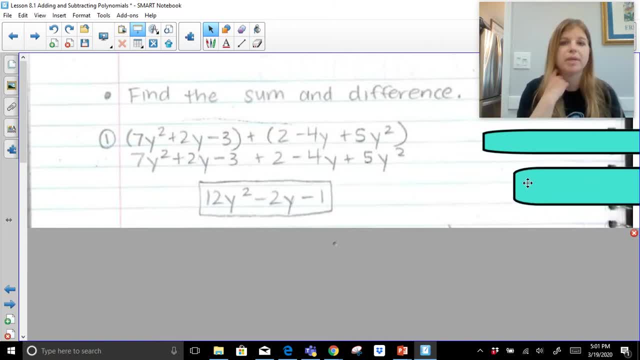 3 and a positive 2 add up to give me a negative 1.. If I gave you this polynomial, I would ask you what kind of polynomial is it? You would tell me it's a trinomial. If I asked you what's the degree? 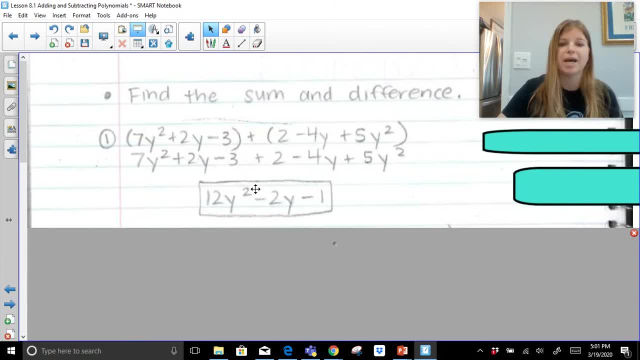 of this trinomial, you would say it's 2, because 2 is the highest exponent. And if I said to you what's the leading coefficient, the leading coefficient is 12.. It's the coefficient of the first term in standard form. Now we're going to take these two trinomials and, instead of adding 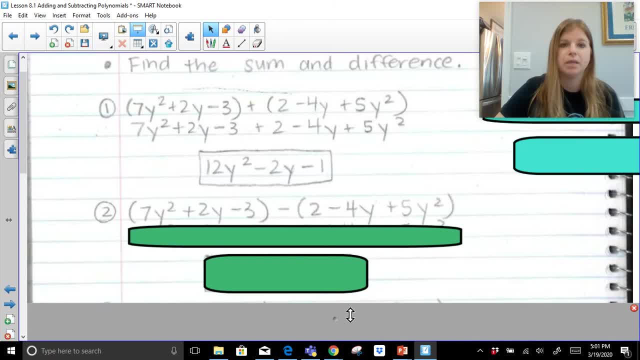 them. excuse me, we're going to subtract them. We're going to find the difference So you can see they're identical to each other. I just changed the plus sign to the minus sign and you're going to see I do that in the next few problems as well. 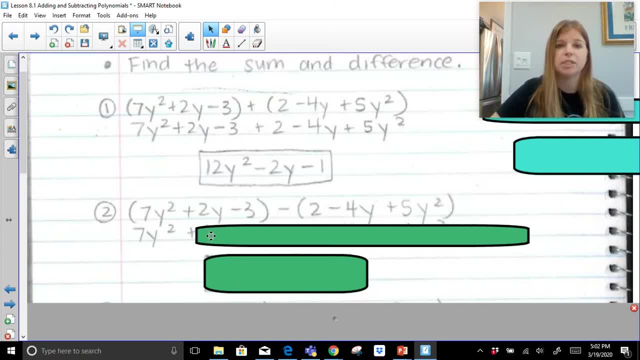 When we are subtracting the first set of parentheses, which is grouping those three terms together is kind of unnecessary, But the second set of parentheses is incredibly important. What we need to know is that we're not just subtracting 2,, we're also subtracting a negative 4y. 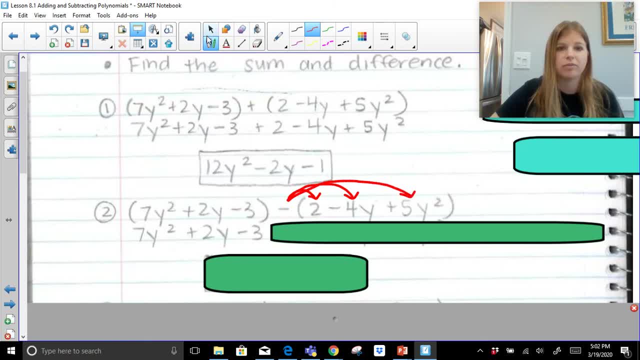 and we're also subtracting a positive 5y squared. So if we know that that we're really subtracting everything, in the second parentheses it's really using the distribution of property, which is what my arrows should really kind of indicate to you. If I'm subtracting 2,, 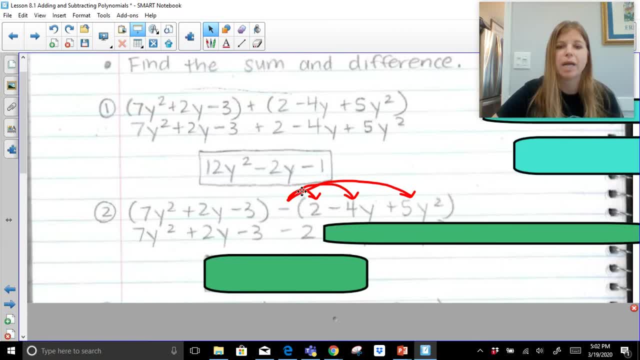 that really means minus 2.. If I'm subtracting a negative 4y, that means I am adding 4y, and if I'm subtracting a 5y squared, then I'm really subtracting 5y squared. Notice: 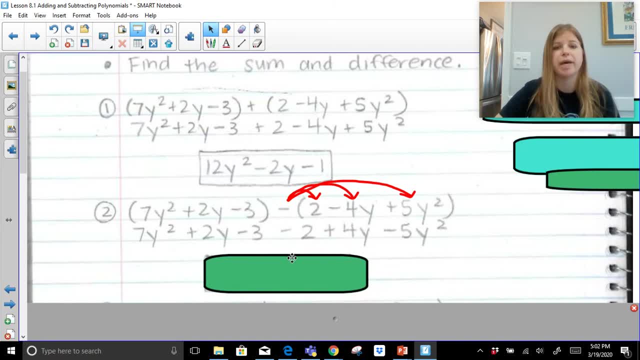 I never told you to bring down any signs. I never tell my students to do that. You simply distribute and bring down your result. distribute and bring down your result. Now we have to combine like terms in standard form. So we work with our highest degree, which is still exponent of 2.. 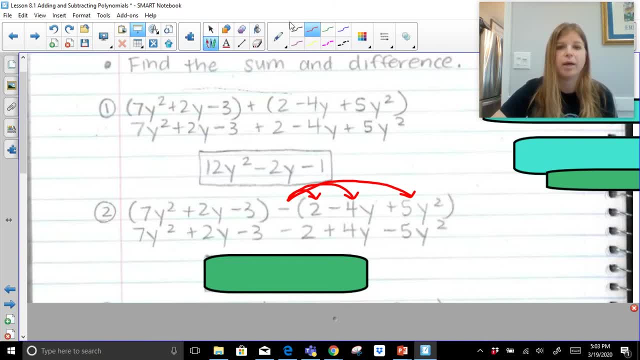 7y squared and a negative 5y squared, and just to kind of guide us along, I'm going to underline them. A 7y squared and a negative 5y squared would combine to give us 2y squared. A positive. 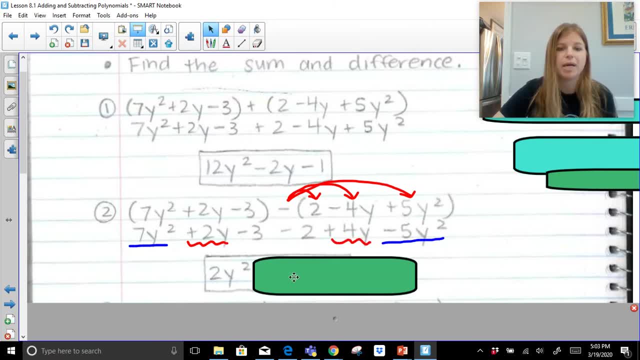 2y and a positive 4y would add up to give us 6y. And then, lastly, a negative 3 and a negative 2 combined to give us a negative 5.. What kind of polynomial is our result? A trinomial. What's the degree of the trinomial 2. And what's my leading coefficient? 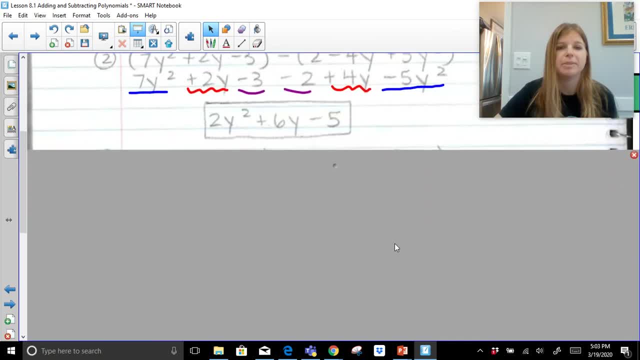 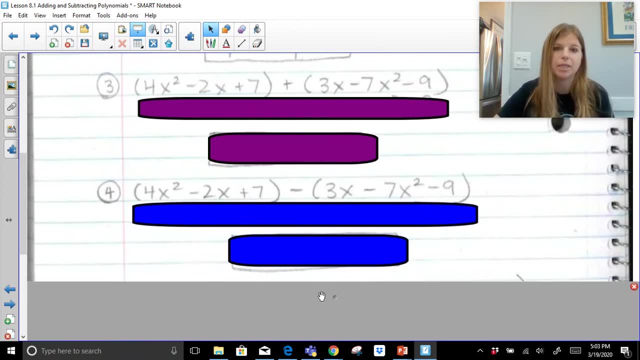 It's also 2.. Next set of problems: Same concepts, guys, Same concepts. We're going to take two trinomials, we're going to work on adding them and then we're going to work on subtracting them. 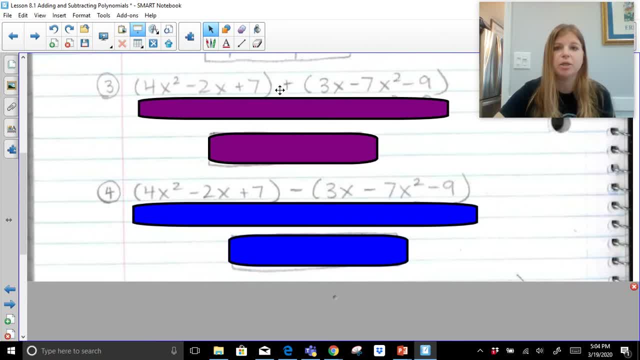 So what I told you before in the first problem is that when you're adding polynomials together, parentheses are irrelevant. They don't mean anything. So I'm going to go ahead and I'm going to rewrite this expression without the parentheses, because they're really just grouping terms. 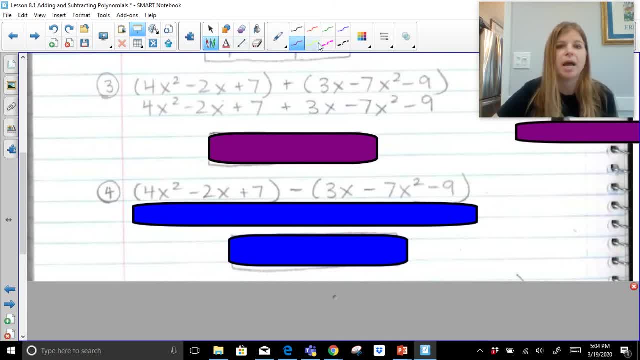 together, which aren't really necessary here. I now want to combine my like terms in standard form. so the highest degree to lowest degree, A: 4x squared minus 7x squared. 4 minus 7 is negative 3, so negative 3x squared. Then I'm going to take a look at a negative 2x squared. 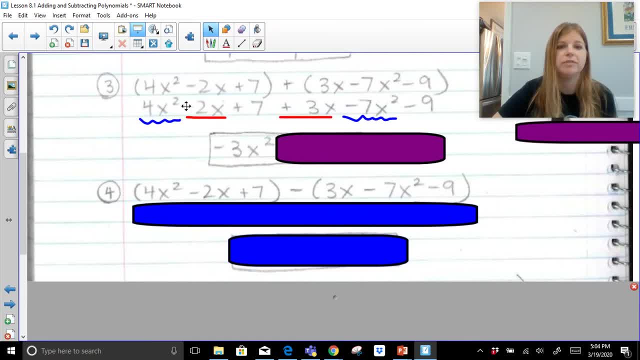 plus 3x. Negative 2 plus 3 is a positive 1x. And then, lastly, I'm going to take a look at positive 7 minus 9,, which is negative 2.. This is again a trinomial. It has a degree of 2, and my leading 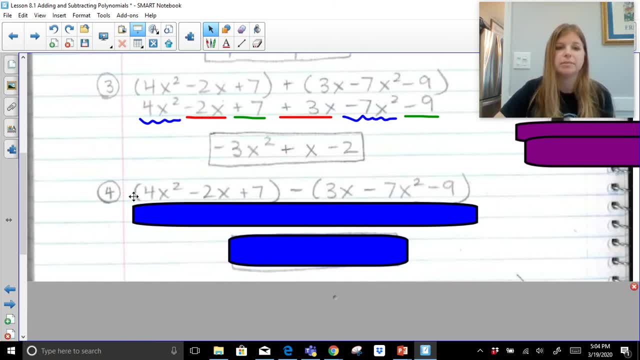 coefficient is negative. 3.. Subtracting First parentheses can get dropped, Just the first one. It's not important, It's not really helping us with anything. We want to make sure that we're distributing our negative. So if we're subtracting a 3x, 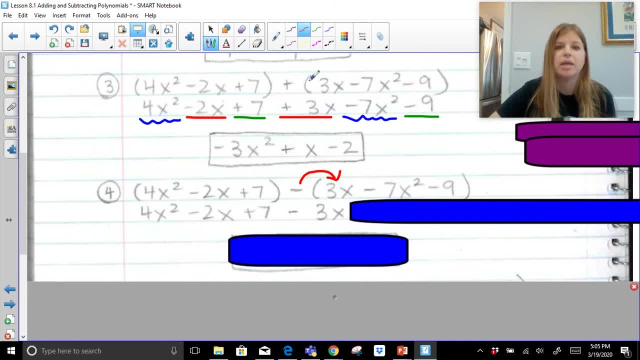 that really means we're doing minus 3x. If we are subtracting a negative 7x squared, that means we are really adding 7x squared. And if we are subtracting a negative 9, that really means we are adding 9.. So now 4x squared and a 7x squared combine to give us: 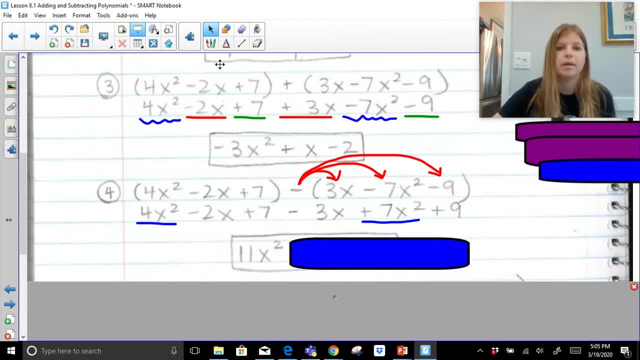 11x squared. Negative 2x, negative 3x- Always notice I put the sign with that term- Negative 5x. And then, lastly, we have a positive 7 and a positive 9, which give us 16. I have a trinomial degree of. 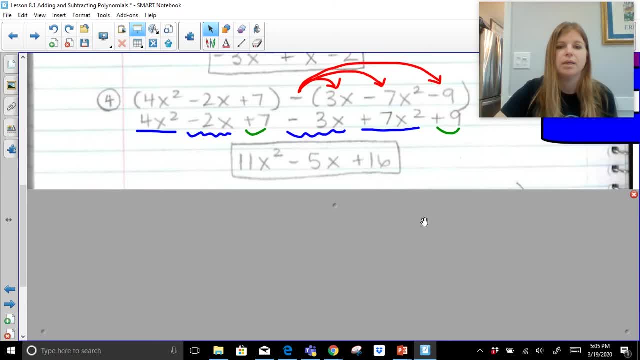 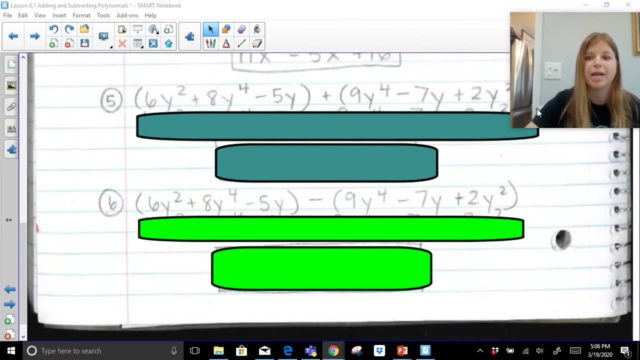 2, leading coefficient of 11.. Last two problems for us today: Okay, same idea. We're going to be adding these Trinomials together and then subtracting them. I just need to squeeze myself over into this corner. So if I'm adding these two trinomials together, we know that we can just simply drop. 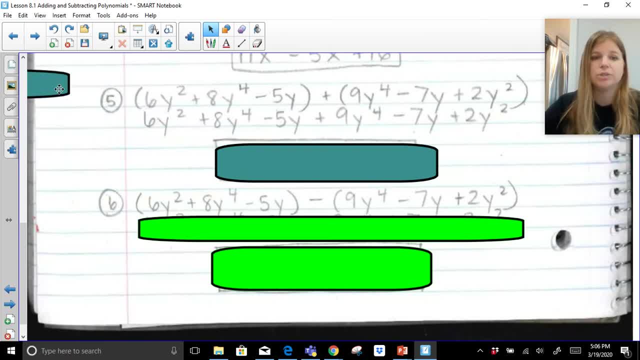 our parentheses. They're not adding or giving anything to this problem. We're now going to add them in standard form, So I look for my highest degree. What would you say is my highest degree here? If you said 4, you are correct. So a positive 8y to the fourth and 9y to the fourth. 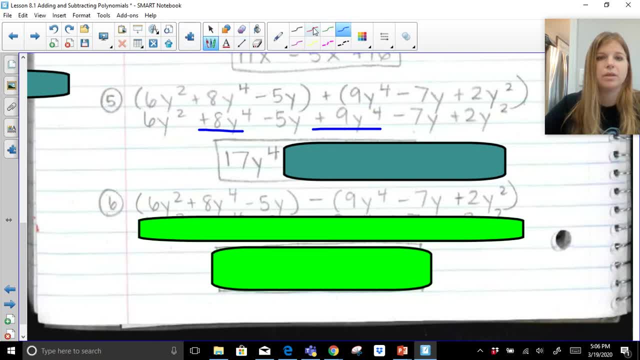 Give us 17y to the fourth. Then I would look at my square: It's 6y squared and positive 2y squared. Give us 8y squared, And then lastly, a negative 5y and a negative 7y. Give us negative 12y. It's a. 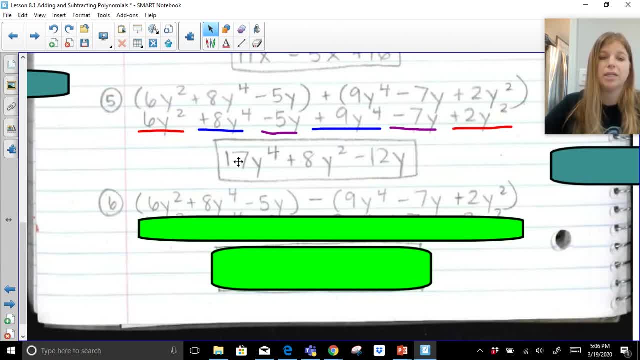 trinomial with a degree of 4 and a leading coefficient of 17.. Last one: we're going to take those two trinomials and subtract them. First set of parentheses can get me 7y to the fourth. They don't really do anything for us. We make sure we distribute this minus sign to each of the. 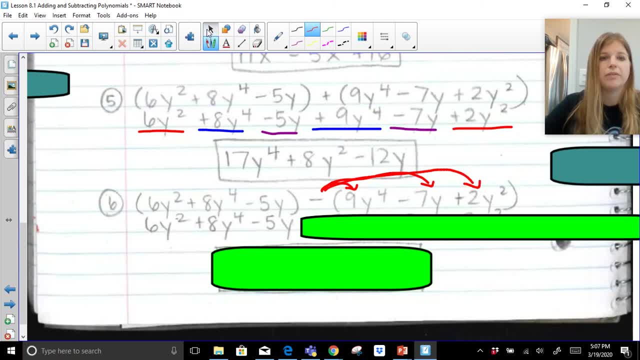 terms in that next parentheses. So if I'm subtracting a 9y to the fourth, then if I'm subtracting a negative 7y, it really means I'm adding 7y, And then if I'm subtracting 2y, squared. 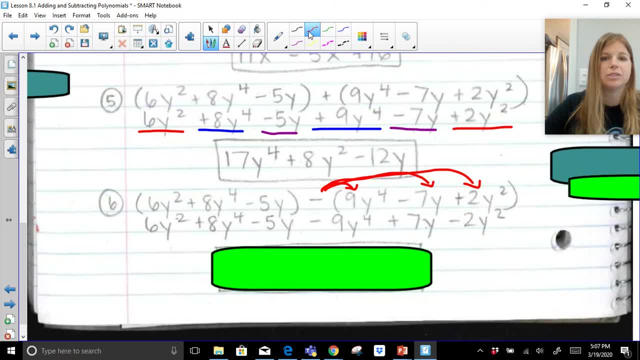 again, I'm subtracting 2y squared. I'm going to combine my like terms in standard form. So positive 8y to the fourth Minus 9y to the fourth would be negative y to the fourth, really negative 1.. Then I'm going to look. 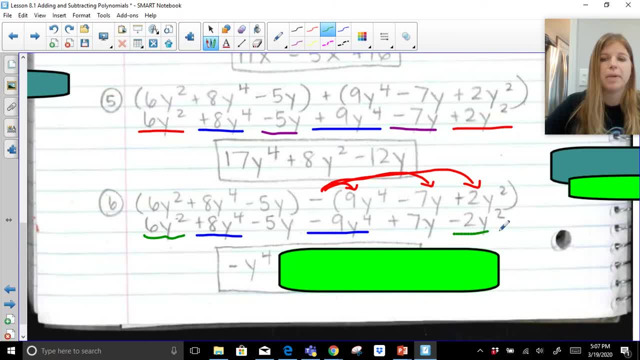 at my next set of terms: 6y squared minus 2y squared, which gives me 4y squared. And then, lastly, I'm going to take a look at negative 5y and positive 7y, which would add up to give me: